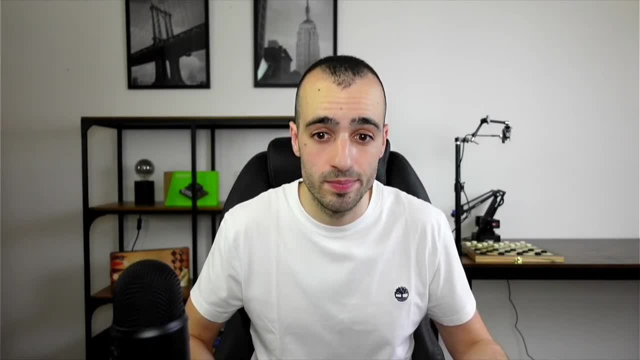 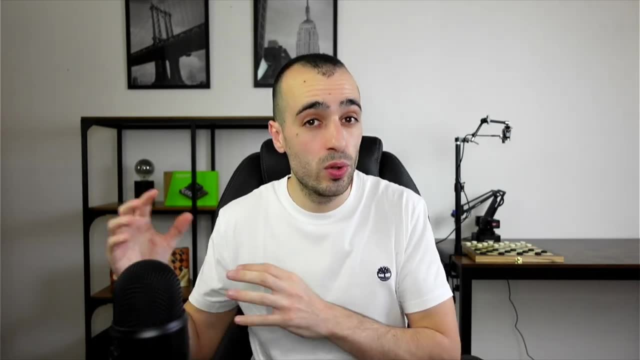 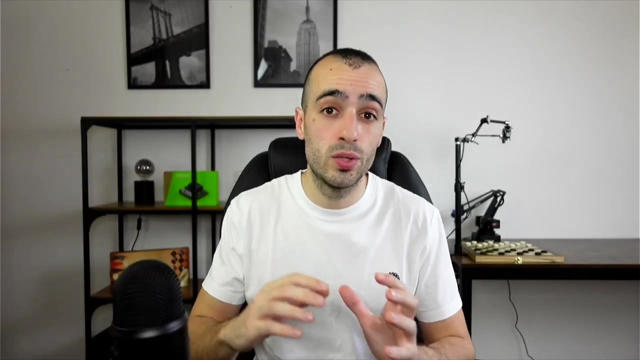 intelligence that plays checkers with a robot arm. Why did I come up with such idea? Well, I wanted to bring something that shows how we can integrate computer vision into the real world. so bringing the robot arm together with computer vision and some game seem a 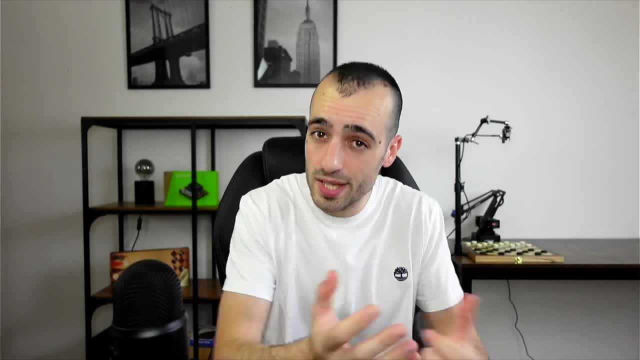 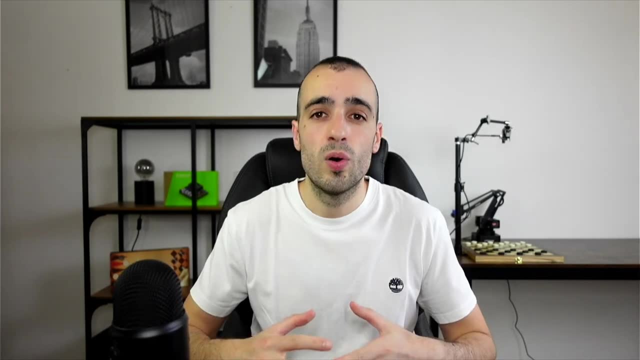 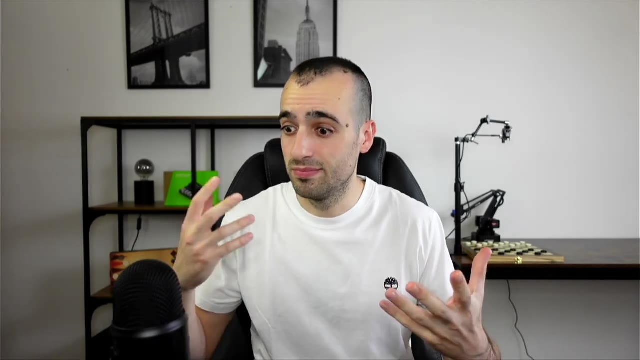 lot of fun and also very useful to give you a perspective of what you can do with computer vision. We're going to see all the challenges that I've been facing while building such project. I will show you all the steps that I used that took me to build this, not only the computer. 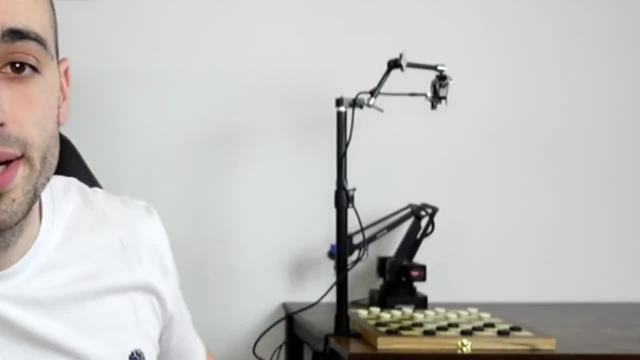 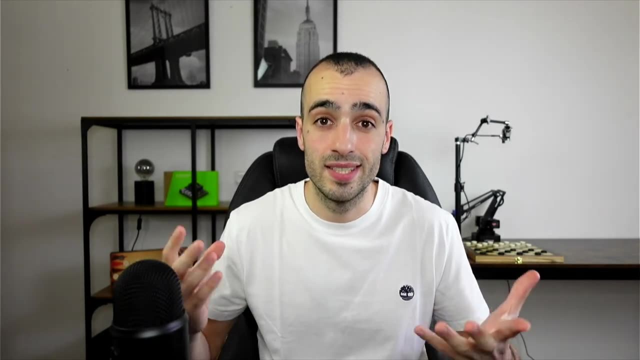 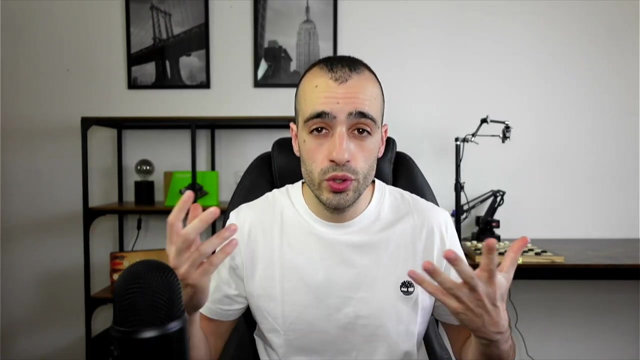 vision part, but also the robot arm part. We will see the hardware that I've been using and the struggles and the successes that finally, hopefully, I got, and you will see that as well. Before starting with this project, I want to let you know that whether you're a developer, you work in a company or you are. 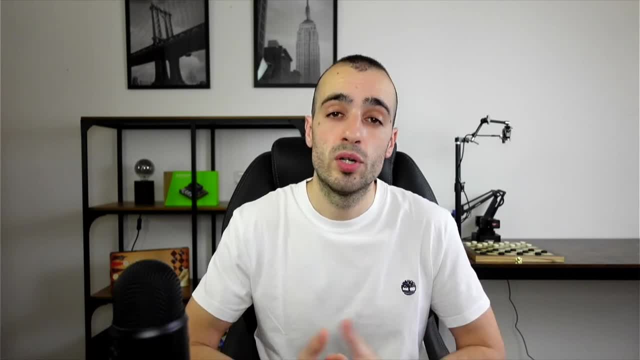 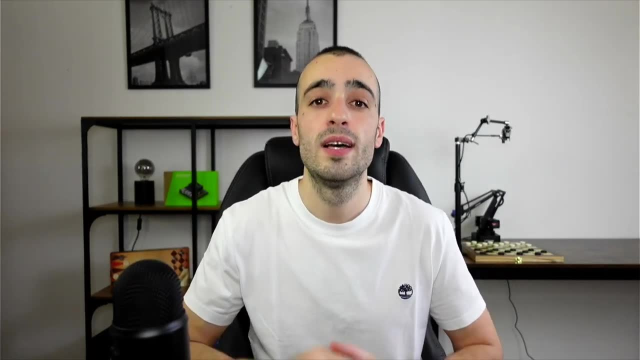 just a beginner and you want to learn more about computer vision, even if you don't know where to start? I have a free crash course that you can download from the link down below by Pysorcom slash blueprint. It's a one hour crash course where you're going to learn how. 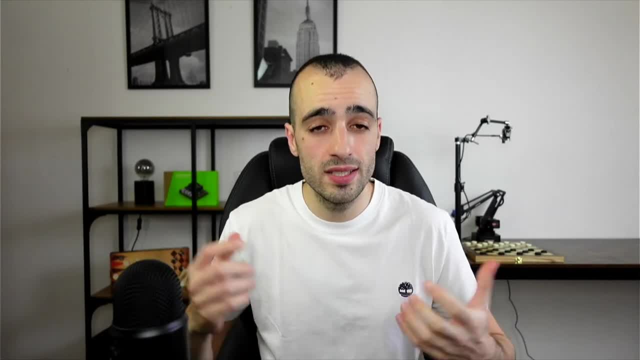 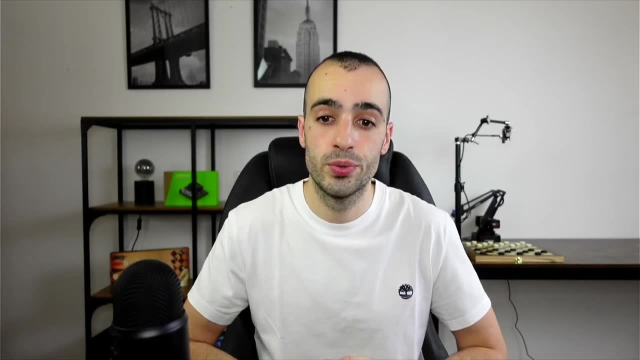 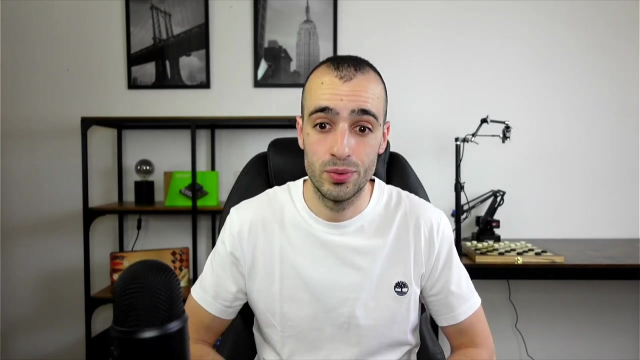 to detect and track any object in the fastest and most efficient way, and I've been using some part of that specific course Later to build this project, because we have a lot of things to detect inside the checker, to get their position and then later, of course, to play against the computer. 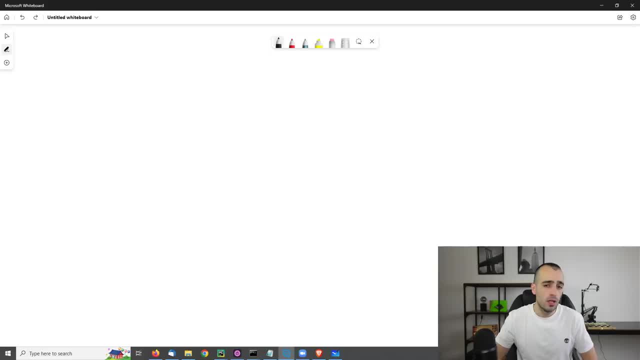 Let's start now with all the steps and let's see. when I first came up with this idea, already knew somehow how I would go to finally build it. and it will require three things, Mostly first one, computer vision. So let me draw like a very rough draft of what I mean with this. 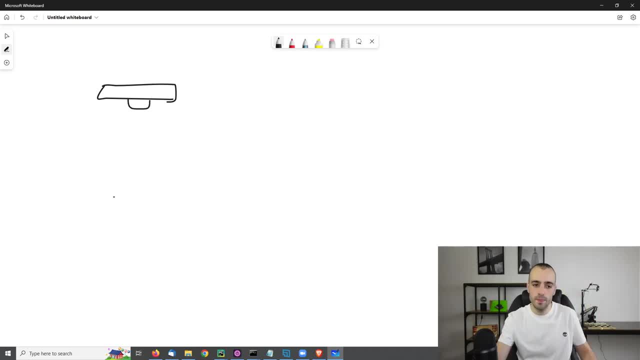 So this would be a camera. Let's say that this is a camera. The camera sees the checkers, just to give you an idea, where the blacks on one side and the whites on the other side. the camera will see them through computer vision. So let's say the camera will see them. 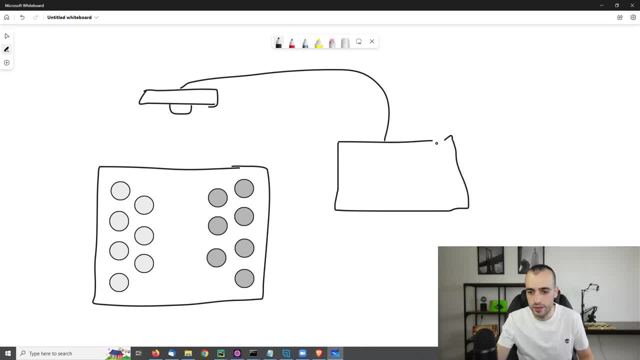 This is: This is connected with computer vision. so with computer vision- comp vision- we will detect them and then we will bring these to an AI which knows how to play checkers, and the AI will be connected to a robot arm and the robot arm is going to pick the object from. 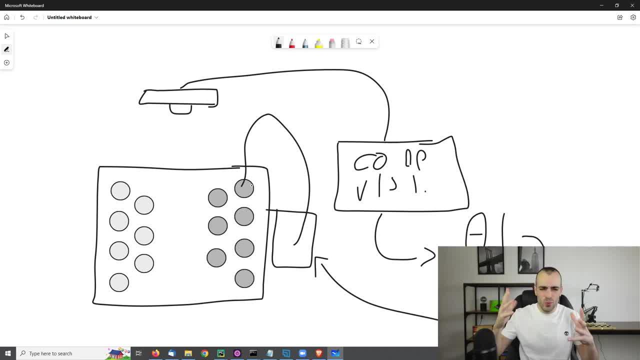 The position makes all the movement, So we need somehow to integrate a few things between them to make everything work correctly. So it's easier said than done, because there are a lot of things which could go wrong if you don't don't do the things properly. 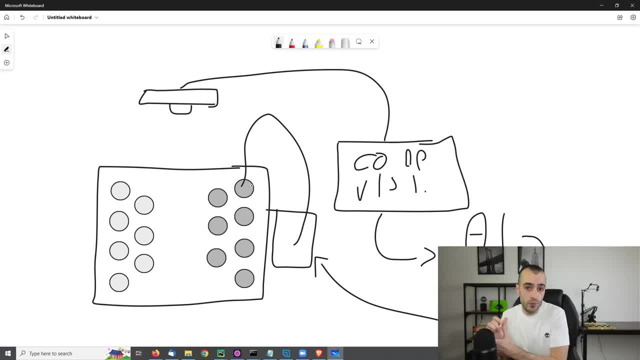 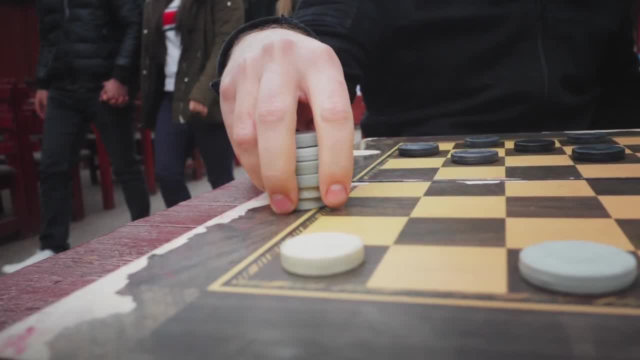 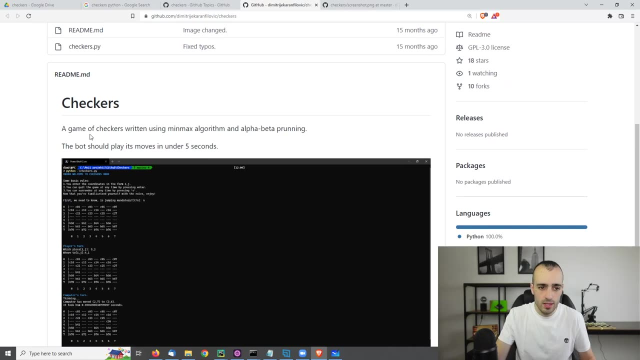 The first thing I've been doing was to look if there was some already simple to integrate artificial intelligence that could play checkers. I found a few of them, But I want to show you the one that I got, So I've been using these specific GitHub project. 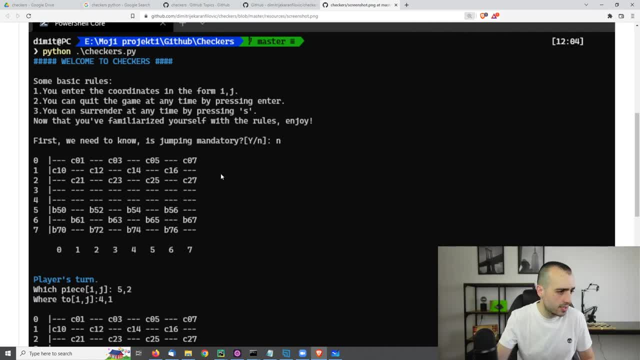 Let me see if I can increase the size of this image. So this is a Python code that can play checkers, and it's only with the code. there is no graphical user interface, and that's great because it makes things much easier later to integrate, because we don't need the graphic. 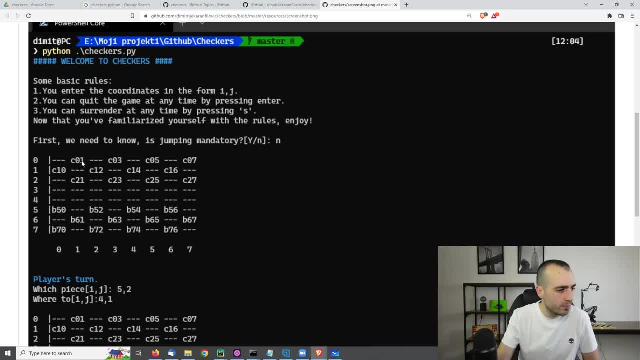 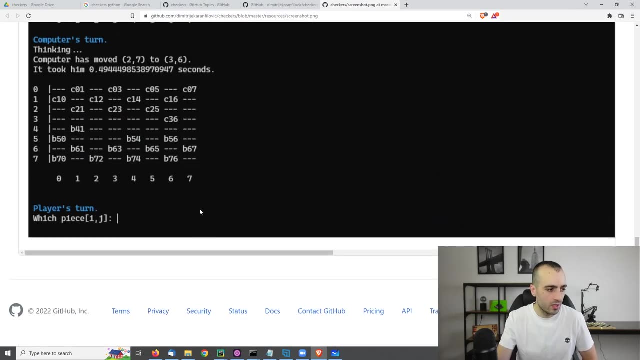 We just have the checkers right here. We have all the position in these metrics that we can see. right here We have, like, the rows from zero to seven and the columns from zero to seven. So we have the starting position and then, once you play, we have the checkers. 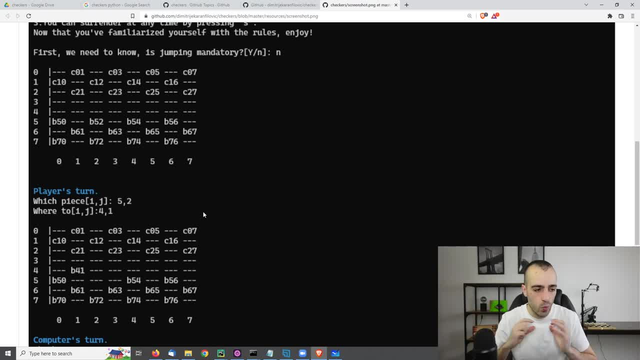 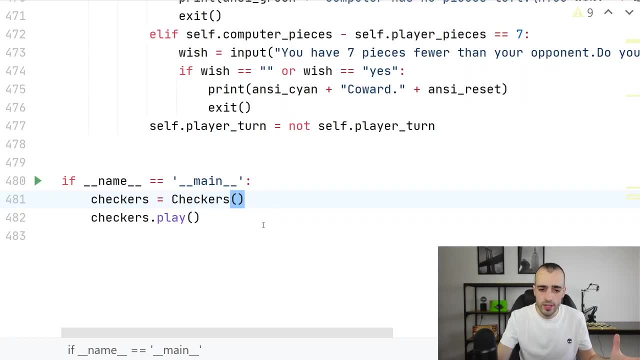 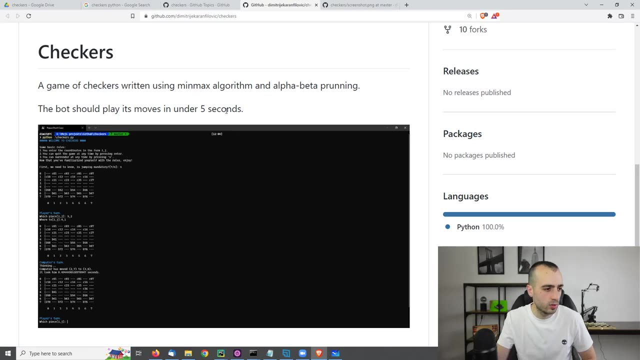 So I'm going to quickly show you how this works and why it's so great this to be later integrated. So let's check this one. I'm not going to run the code I use from GitHub that some developer. Okay, let's first me quote: like the code, and I'm going, by the way, also to put all the links. 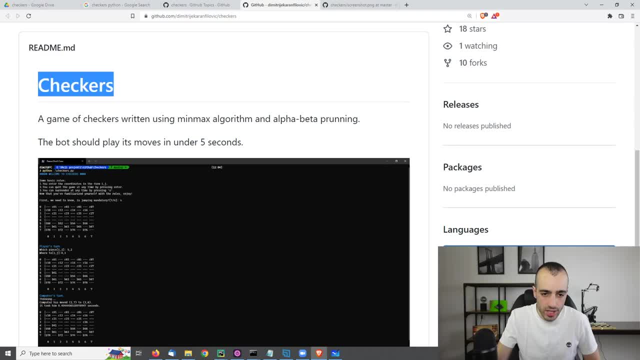 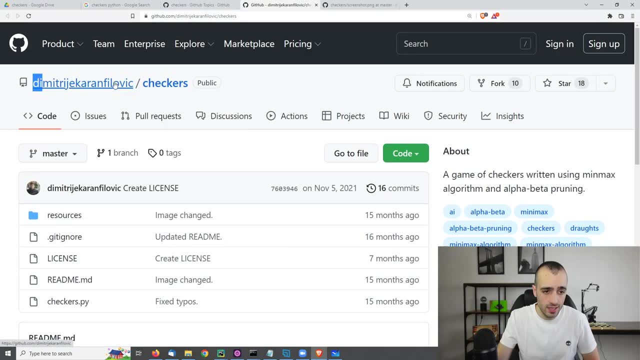 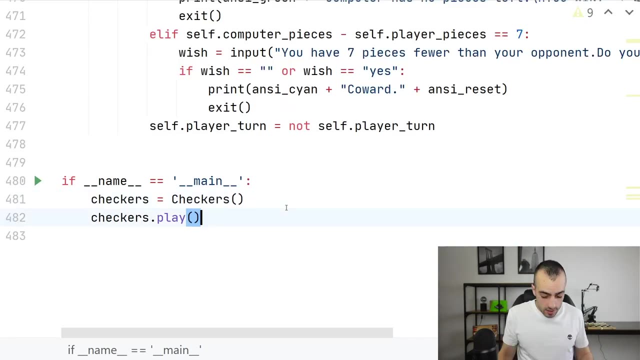 down below on the blog post. So this is a checker that plays with AI and it makes a move in under five seconds by Mitri Karan Filovic. Link will be in the description. Let's run now this code right here And let's play with it. 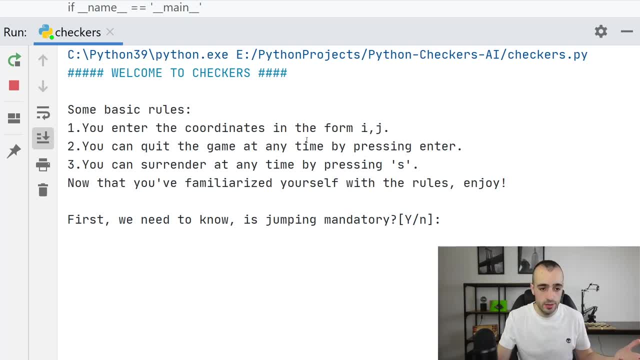 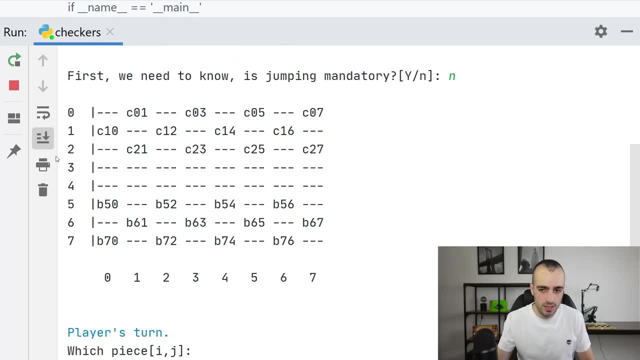 You will see first the rules to play checkers. You can enter the coordinates, We don't really care, because later I will change this code. So let's now just play quickly. Jumping is not mandatory. This is the computer and this is the user. 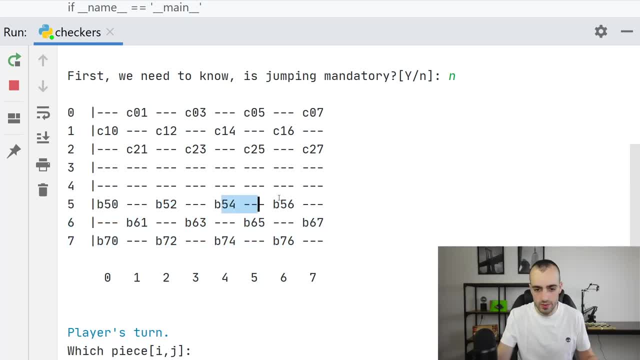 So these are where my checkers position are, which is, of course, the starting point. Now it's player turn. We want to move something, Let's move B 50.. To the position for one, which is this one. So B 52 for one. 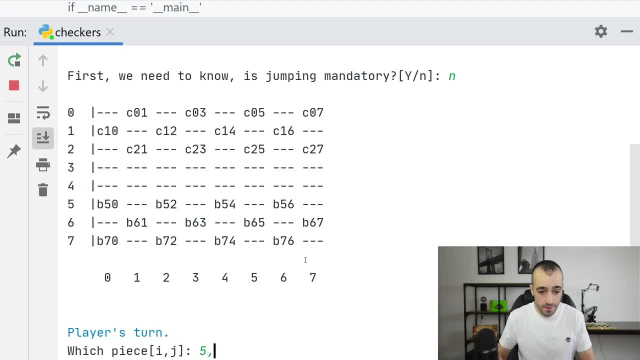 So which piece we want to move? want to move the piece five zero to the position four and one. So we see our position is here and it's very quick, Just right away. It replied. the computer moving to the position See three, six. 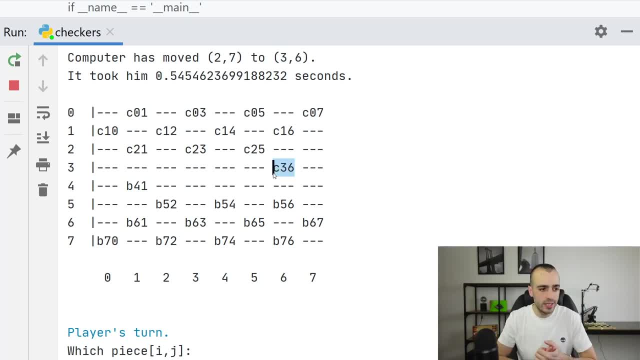 So it moved this one right here. That's enough that we need to know about this game Because it's very easily later to- I mean, is it to some extent um to integrate later this metrics, we the computer vision software, in order to replicate these on the real scenario? 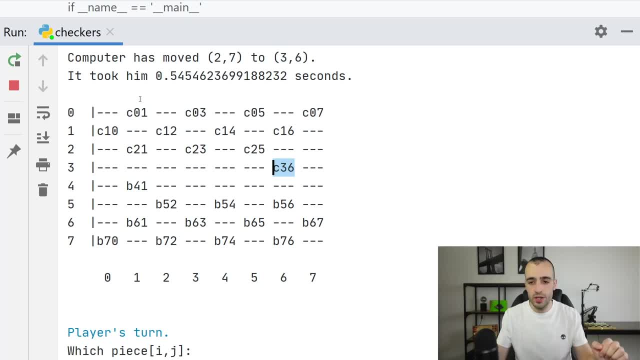 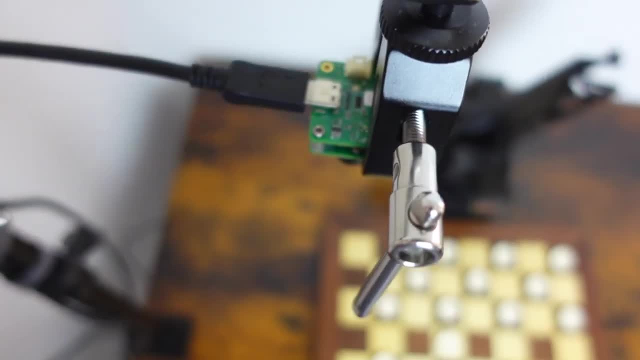 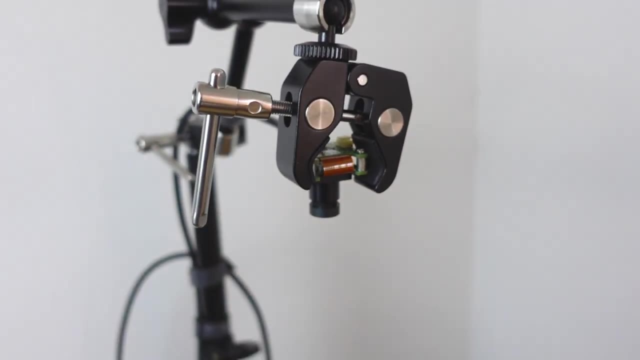 right there. So this was the first move We had. the checkers game is working very well. That's all that we need, And also not about the hardware. I've been using industrial camera, USB industrial camera. the company ecosystem sent me to test, and it's holded by a clamp holder. 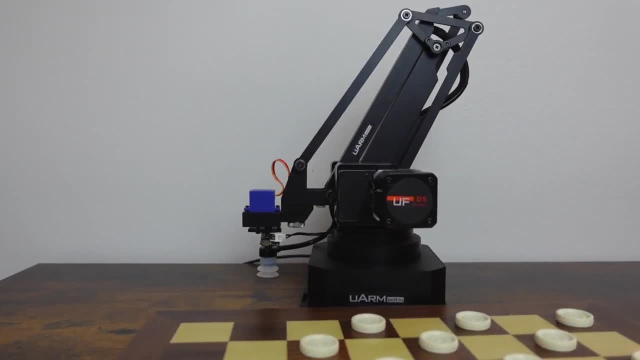 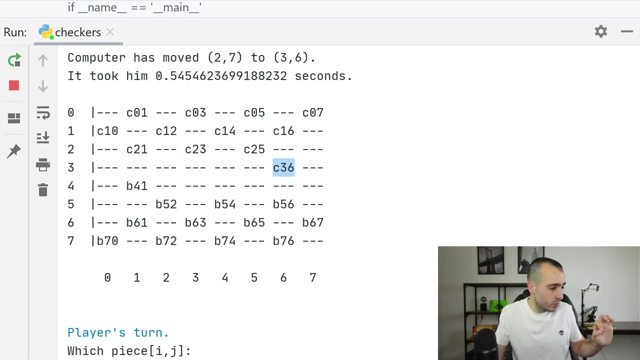 As you can see right here, plus a simple small robot arm from the URM company. Very good for prototypes. Let's now go to the other step, which is the computer vision part- how to detect what's happening on the checkers and how I went for that. 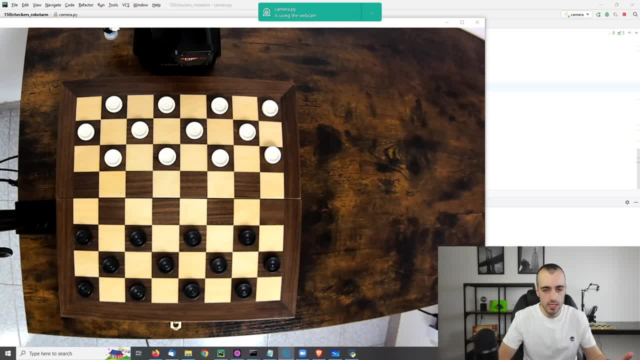 Let's go. Oh, I developed the computer vision part using open CV Mainly, plus some All the libraries for deep learning later. but first I started with open CV. This is what we get from the top camera. So we have a top camera place right here which is getting the view. 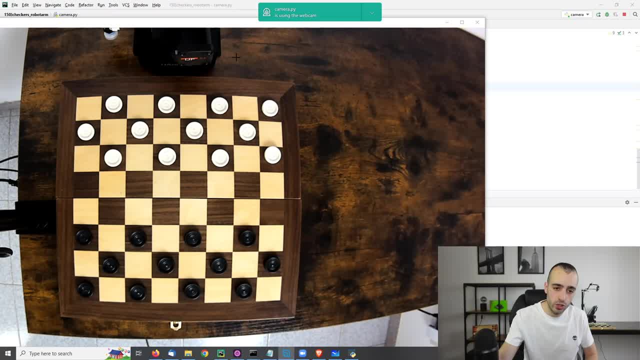 We have only one goal with the camera and computer vision: to detect the position of the different checkers. So of the white ones, we want to know on which specific cell they are located, so that when I talk about uh location I don't know. 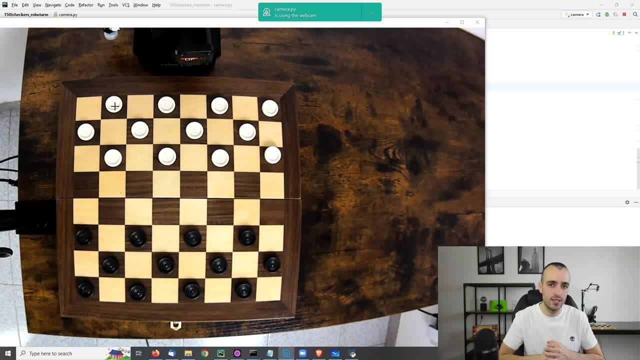 I don't know. I don't mean location in X and Y Z position, because that's more mapping of the robot that we will do later, but it's just simple location on the checker. So the idea is to get the checker separate, the checker in different cells and get the 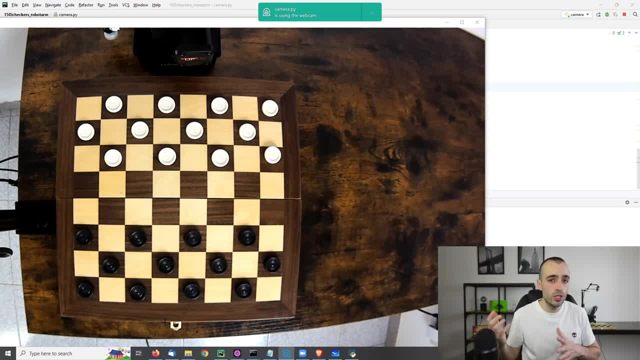 position of the whites and the blacks and see on which cell are they, and make the same as the software for the artificial intelligence. So give a location. For example, this white one on the top left will be position zero one. So zero of the rows, one of the columns. 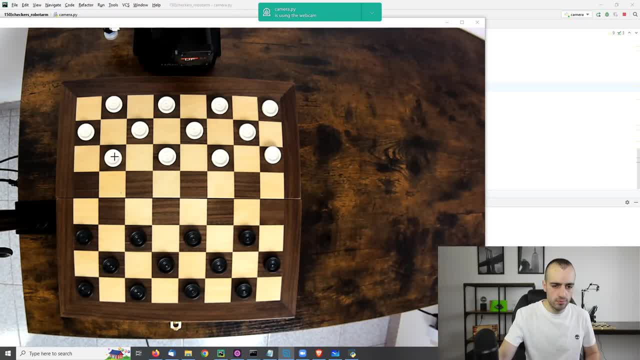 This one will be two, uh one, and so on. for all the other different locations. There are different ways that we can use to detect these objects. Uh, I initially started with something very simple by color detection, Because I thought there is black and there is white. color detection will be quite fast. 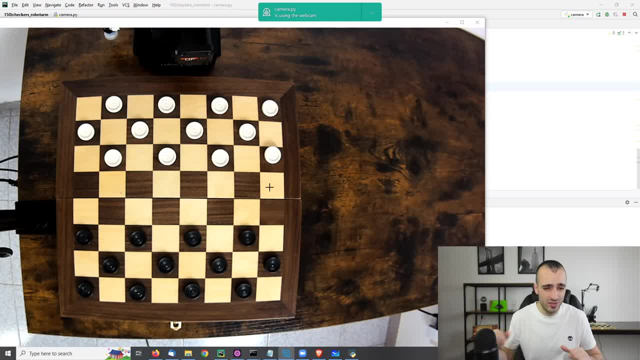 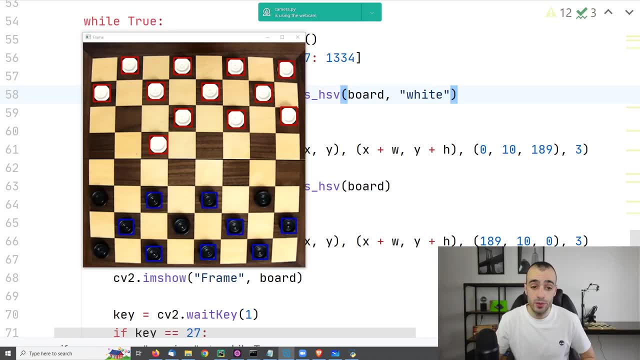 and we can do that. Uh, unfortunately didn't work as well as I expected. Uh, this is the code that I created to detect the checkers based on their colors. So I took some ranges to detect the white and the black. It would work decent, uh, with a specific light. then we've some lightning changes. 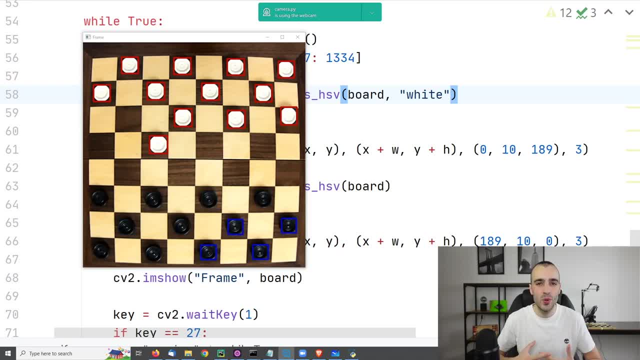 It will give a lot of problems. So I decided to go for something uh, more advanced with deep learning, which was definitely more reliable. You can see that the whites are detected quite well. So if I move them, uh, we have a bounding box, a red bounding box on the white, while 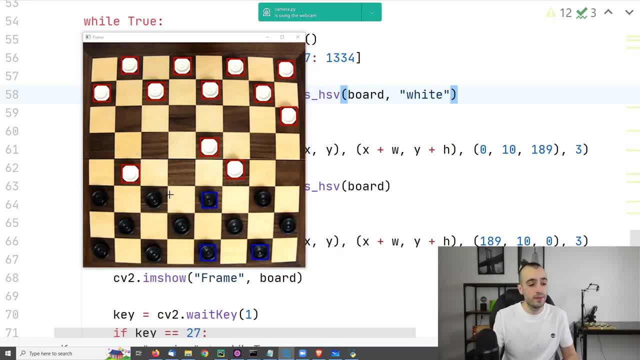 we don't have them for the black And this is very sensitive to lightning changes. So if I change a bit the light, you see we lose some of them And we get them back. This is not reliable, uh, unless we have a stable light. 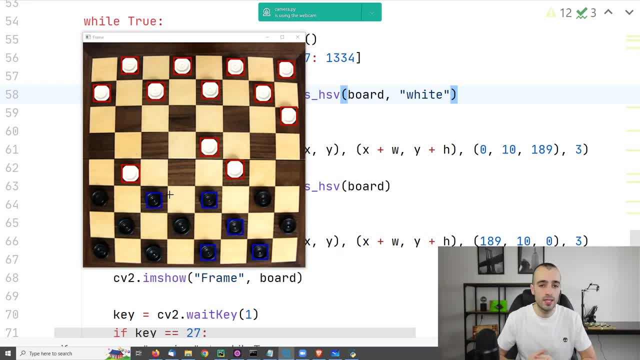 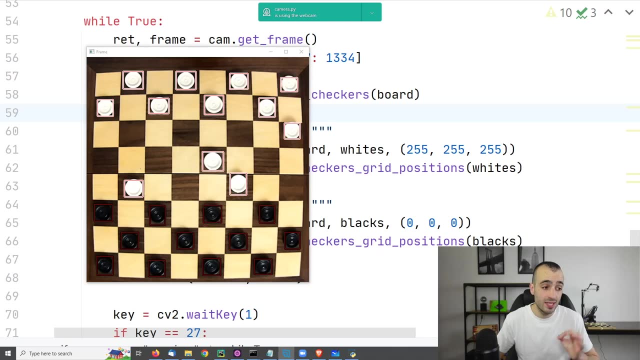 So I opted for deep learning. I created a detector- uh, we uh object detection to detect this. uh, it was working very well with 100% of detection And I'm going to show you that. uh, this one right here is using object detection with. 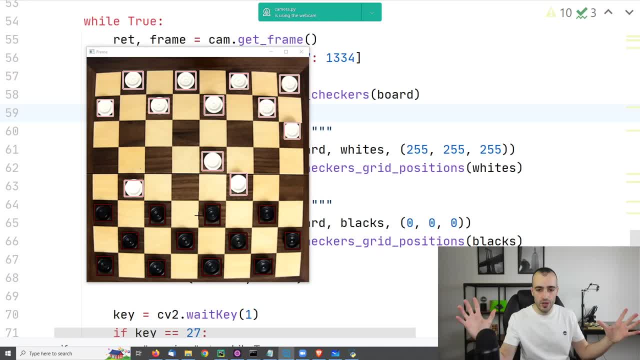 a deep learning, You can see that they are detected very well. All of them are detected, All of them. So if I move them, everything is uh working fine, Uh. I will not go into details about how I created this because it will take very long. 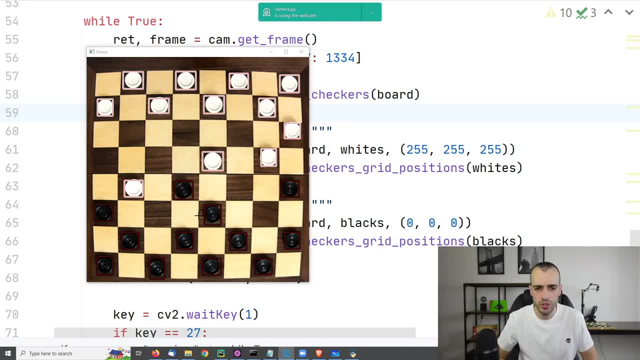 time, but you can check that. uh, on the crash course, I go um about explaining about the different competition method, methods to detect objects, And also I have this and the same exact code to create a detector in my course. Okay, 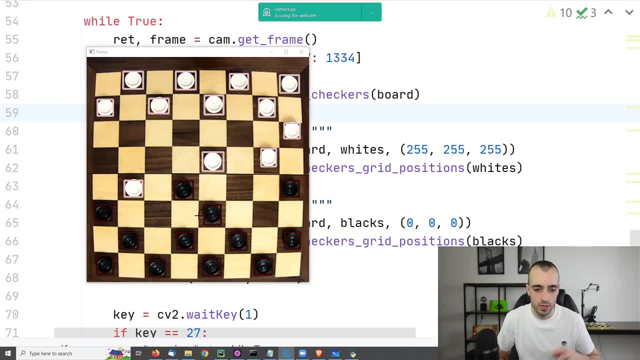 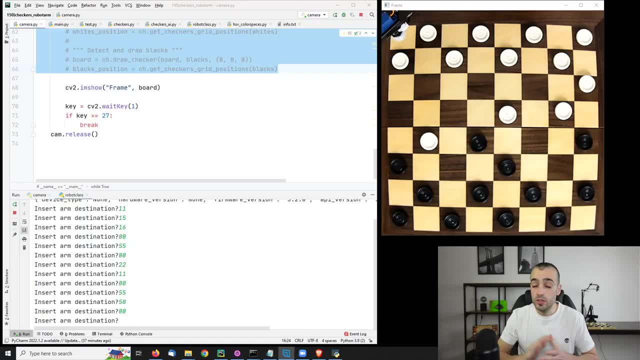 Object action with OpenCV and deep learning that you can find on PySourcecom. Let's now see what we had to do with the robot arm. For the robot arm, I created some simple code which will go to a specific location. We uh, just the output of the cell that I want to take into consideration. uh, as as. 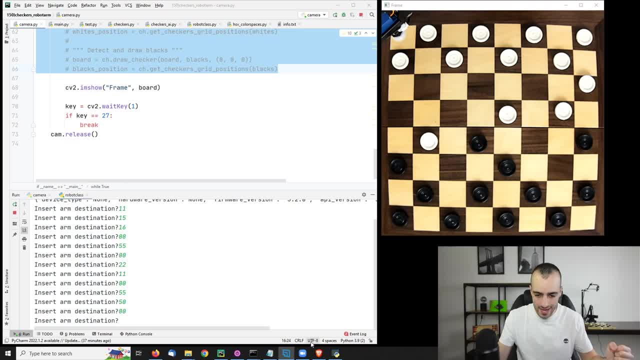 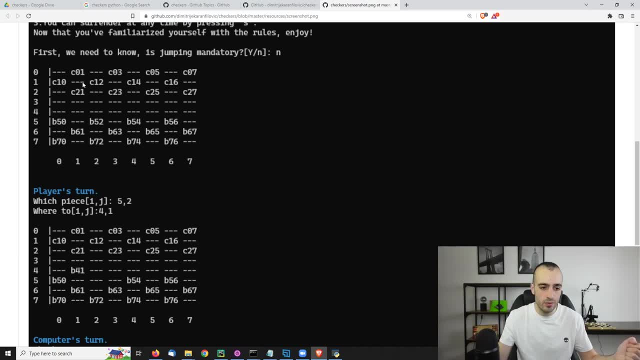 exactly as the software of EAI, This one right here that we use, For example, he. there there is the position 01. right here we say 01 and it will go right there. Uh, let's see an example. 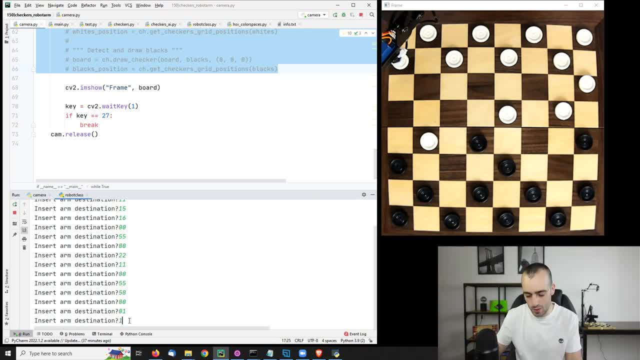 So if it goes 01, okay, this is inverse. So let's say 10, because I use a different system. Uh, I just in inverse the X and the Y, but it exactly the same. Uh, you can see in this example the robot arm which is moving. 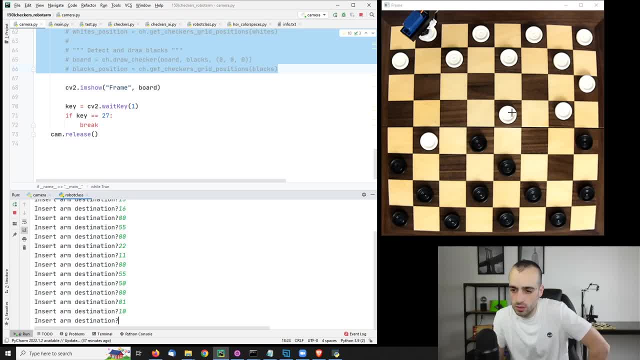 So if I want to move the robot arm, for example, on This white piece right here, it will be one, two, three, four. one, two, three, four, three. So I move, four, three. I just type four, three and we go to exactly that specific location. 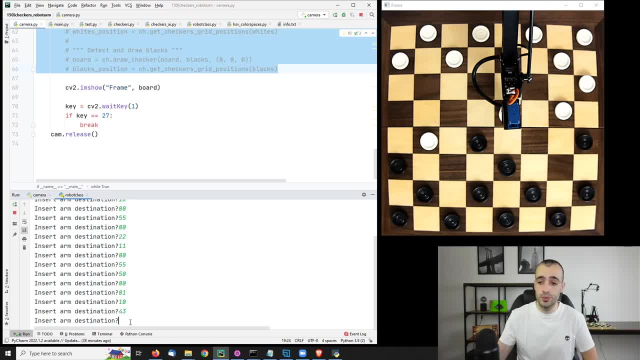 So we have mapped all the cells right here to get that. So if I go, for example, 03 right here, Okay, This way we get the exact location of each of them And, of course, this very basic system and implementation, which doesn't take into consideration if we 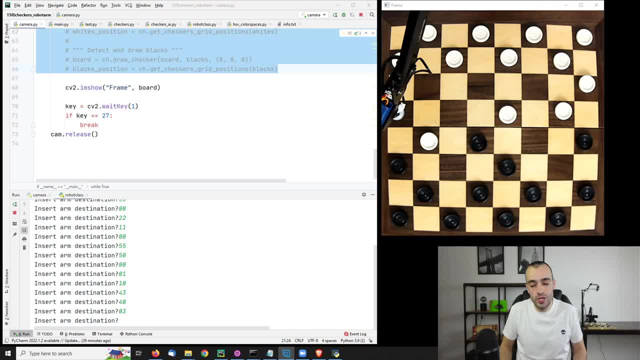 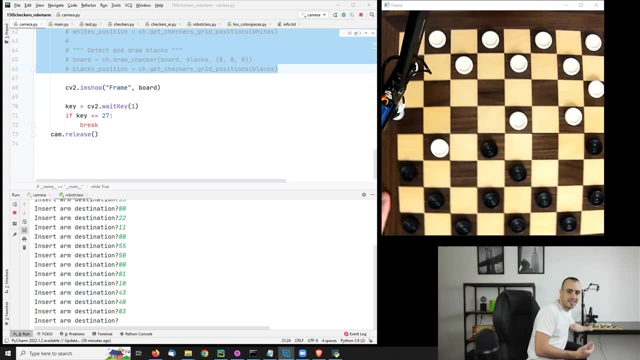 move the checkers away. So we need to have the checkers, of course, into a stable position because we're not detecting native mapping them. uh, from a final view, Let's see an example. If I move the checkers, let's say this way: 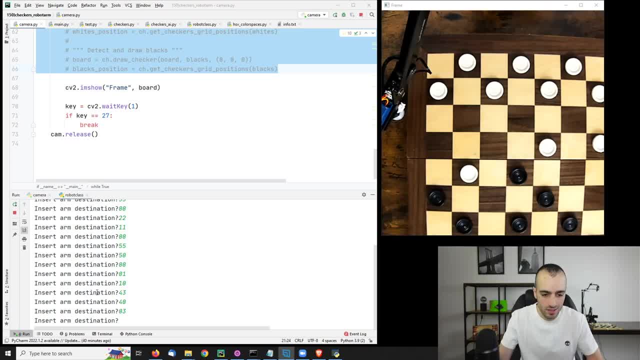 If I move the checker out of the position, it just let's say that I go to, I want to go to 00.. So right here I type 00 and it doesn't go right there. So we have a stable position of the checkers. these very basic concept. 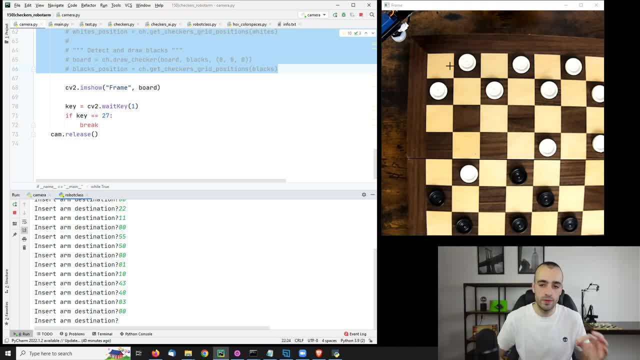 And then uh, all the cells. the position of each cell, uh, was calculated and it's not automatically found with computer vision, Is it possible? So You can find the checkers also when it's moving. So you just place the checker wherever you want to, just put a camera wherever you want. 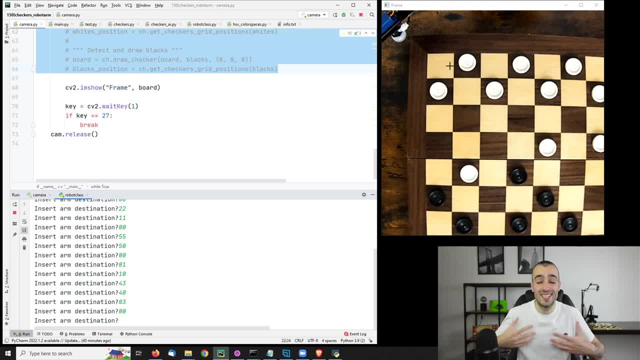 And then you pick the objects. Of course that's possible, but it's much more complex And I didn't want to do that because I wanted to build this project in a relatively short amount of time. So I use the stable position, but you need to know that everything possible right here. 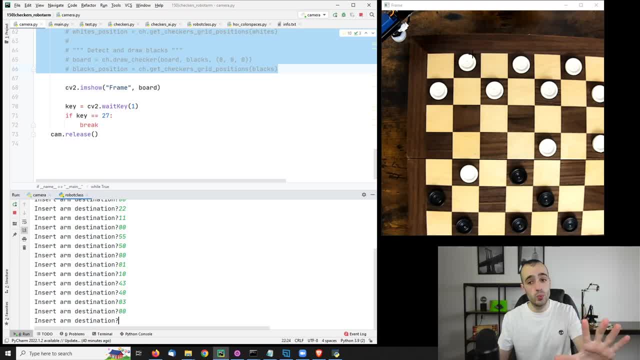 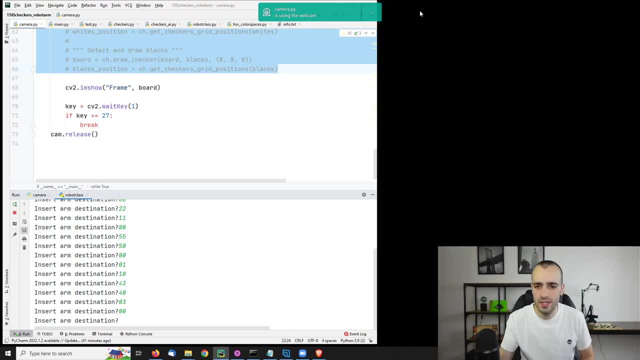 So just that you keep that in mind. So this was pretty much what I had to do with the robot, Um, with something extra, I don't know they they kind of just turned off with something extra, uh, which was to pick the object also. 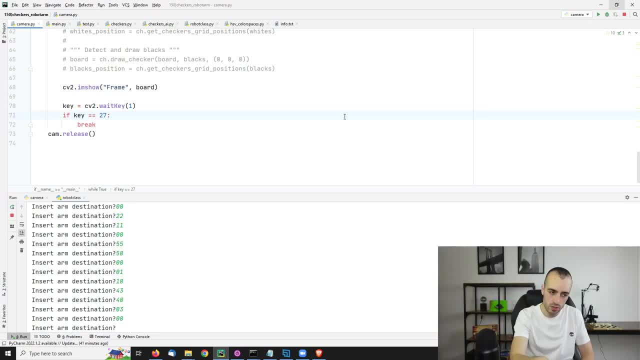 So once we have the position the robot arm needs to go down. So we change some position: go down. We activate the pump to get the checker, brings the checkers to outside of outside to some new uh position. This was pretty much the robot arm. 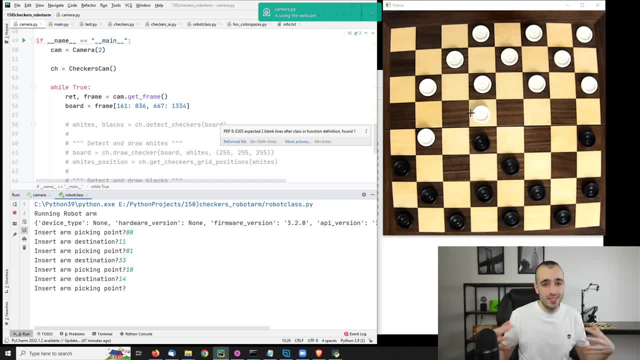 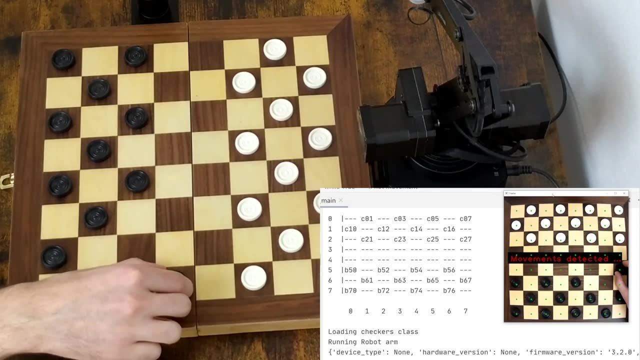 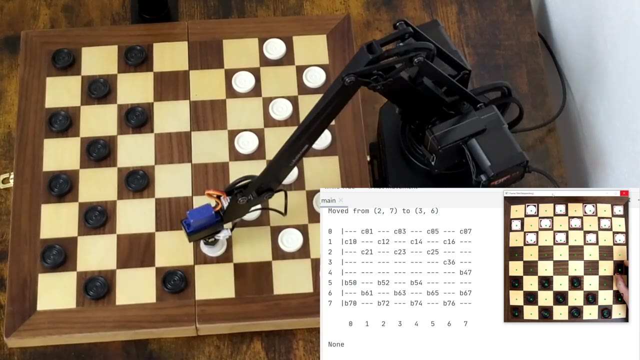 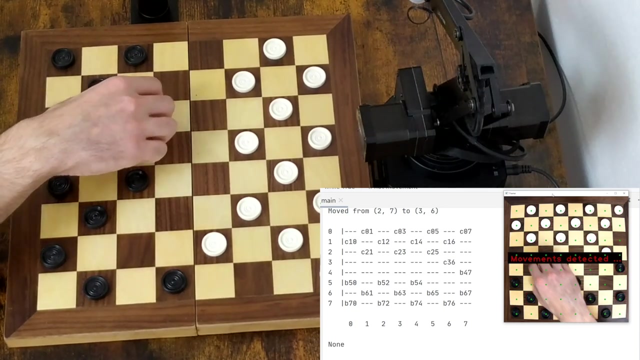 And now The final, most important part is the integration between all these things: the AI that plays checkers, the computer vision and the robot arm. That's the final project. Let's see now how that's working. Yeah, So the 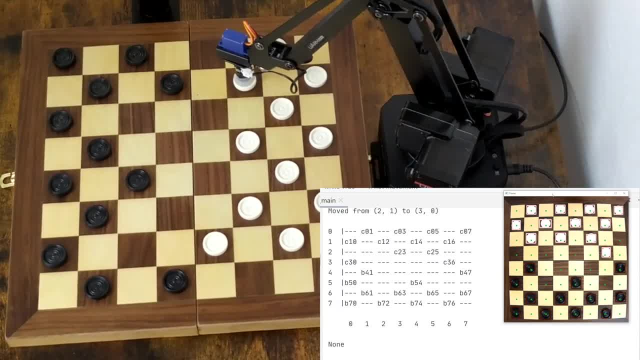 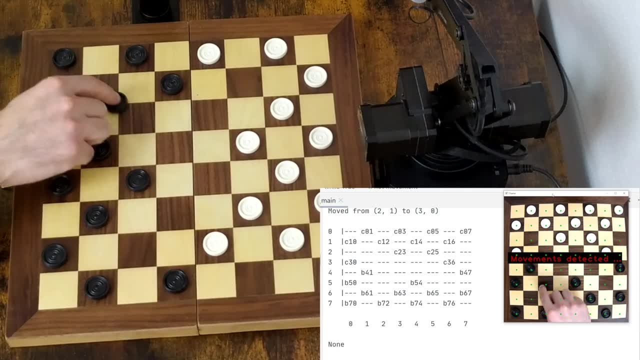 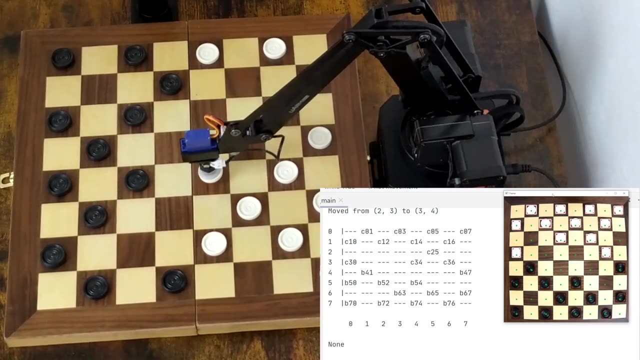 So, yeah, So it's. I'm going to take the voice that's coming from the screen like: and I'm going to take this, this. you know a little bit of a like, an entire thing. We can go ahead and call it back when it's the time to do it. 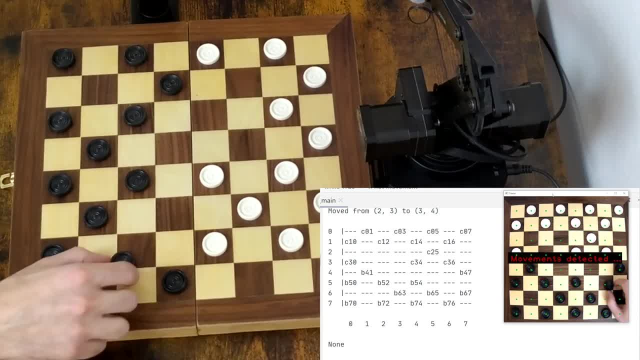 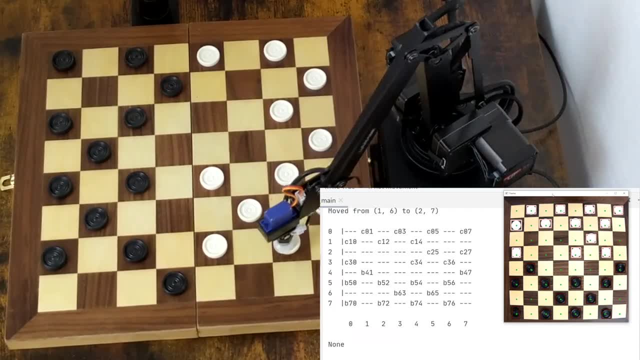 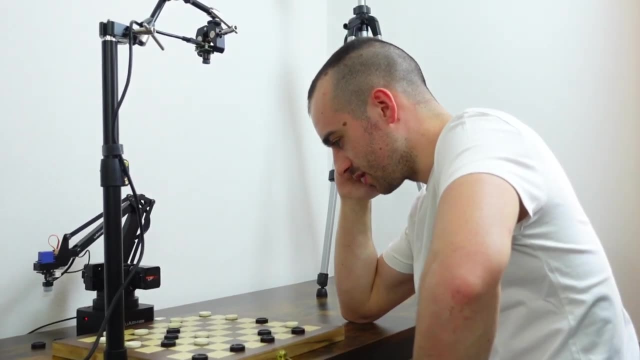 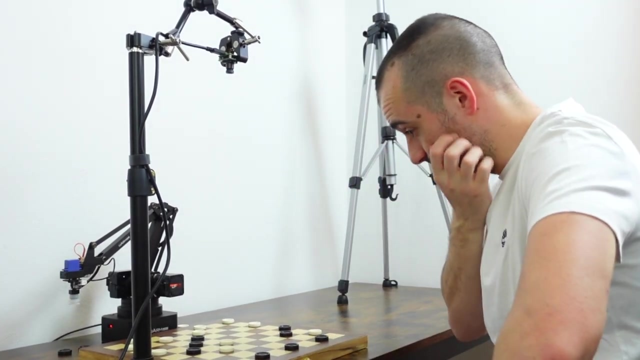 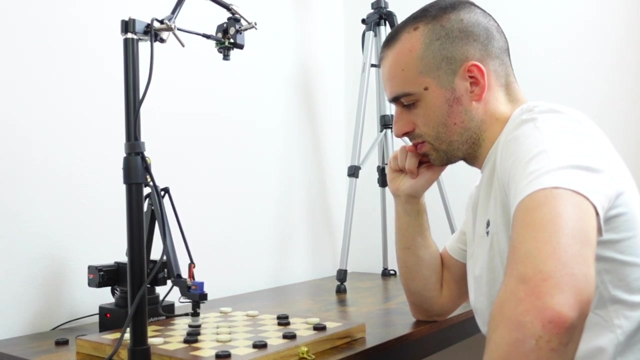 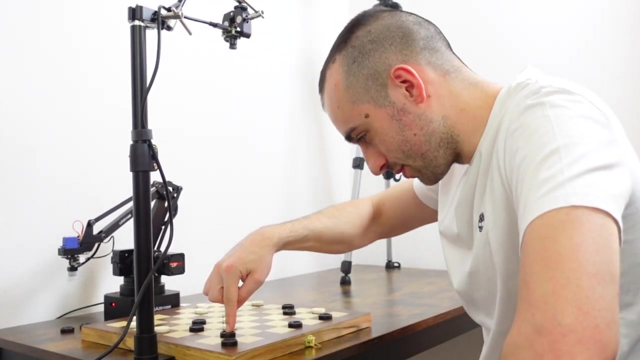 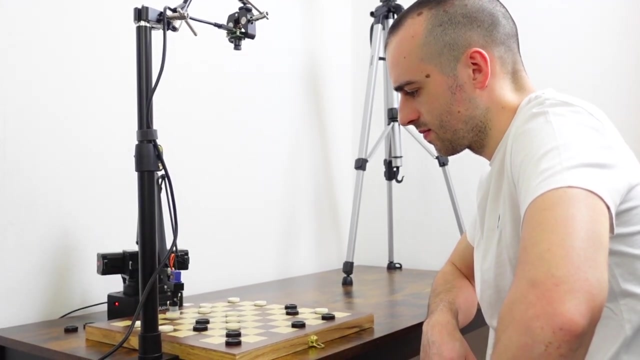 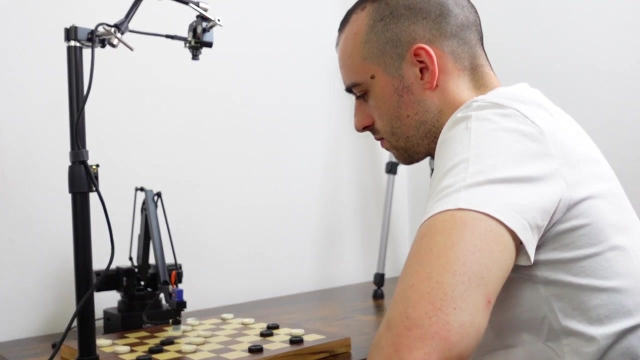 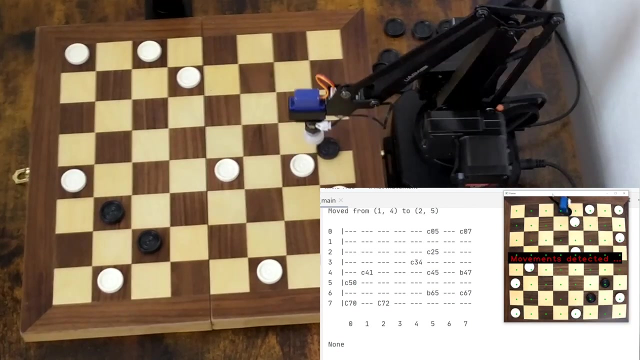 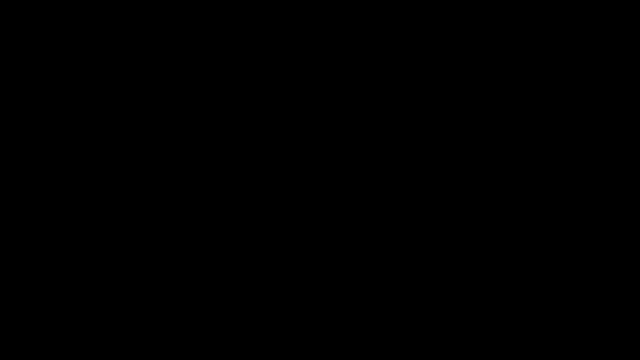 Cool. So the first I'm going to call it. So this is the first thing that we're doing. It's the big, So This is a little bit The. We'll be right back. We'll be right back.